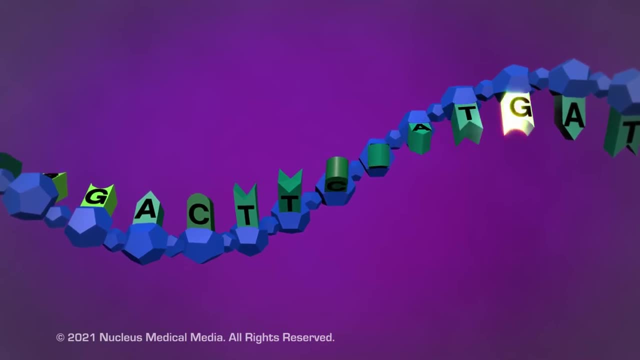 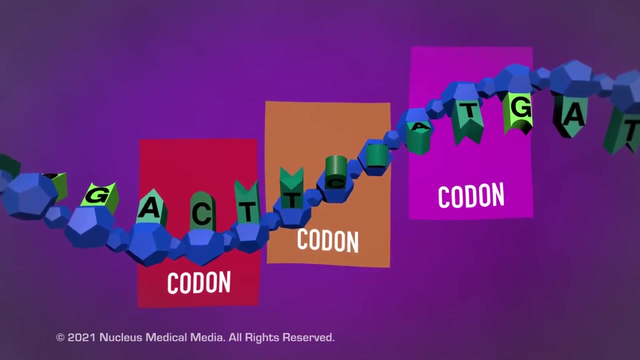 dictates the order of amino acids that will make up the protein. Each group of three consecutive bases in the gene is actually a code for a particular amino acid. As a result, each group is referred to as a codon. RNA polymerase causes a particular area of the DNA helix. 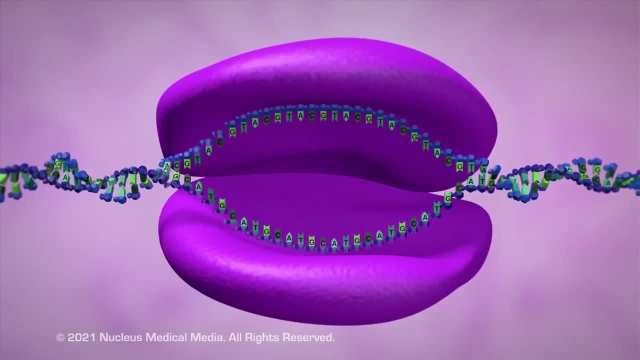 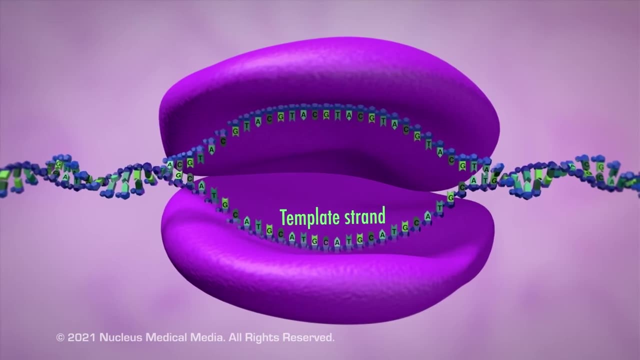 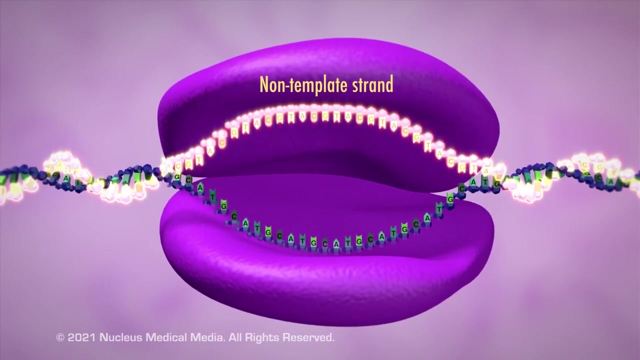 to unwind and separate into two strands. One of the strands, often called the template strand, is the side of DNA that is read or transcribed by the messenger RNA. The other strand of DNA, often called the non-template strand, isn't transcribed by the messenger RNA. 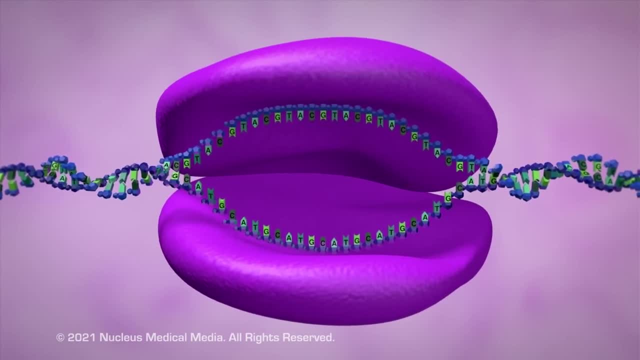 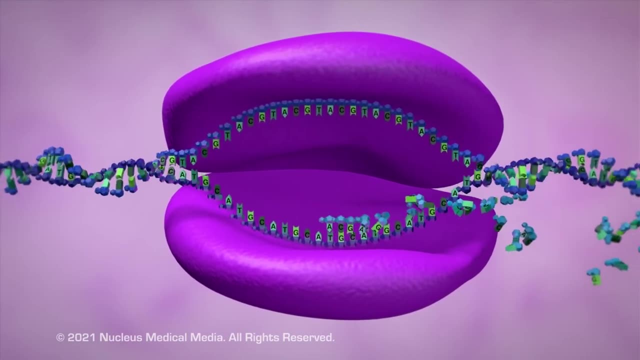 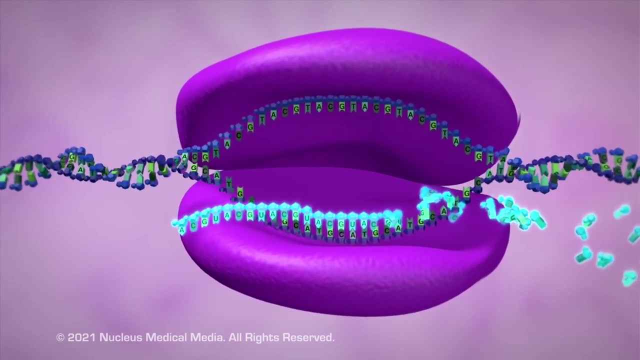 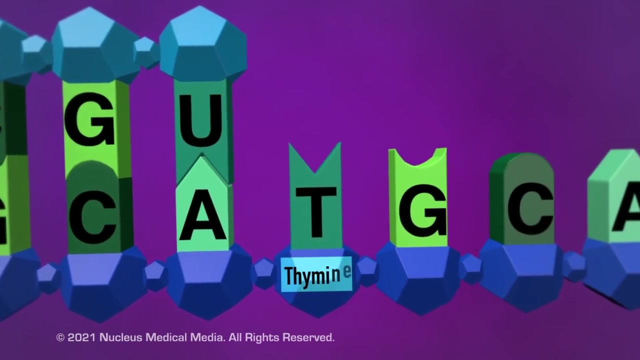 So how are DNA instructions transcribed into messenger RNA? Well, using the template strand as a guide, RNA polymerase uses the base pair rule to assemble free nucleotides in the nucleus into a complementary strand of RNA. For example, RNA polymerase reads the DNA base thymine. 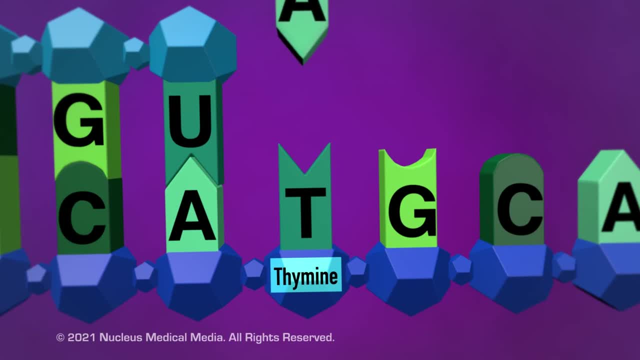 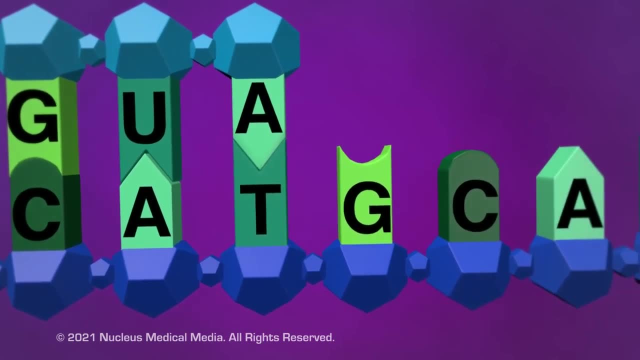 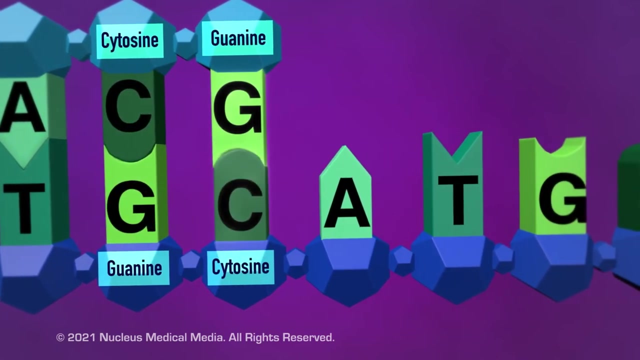 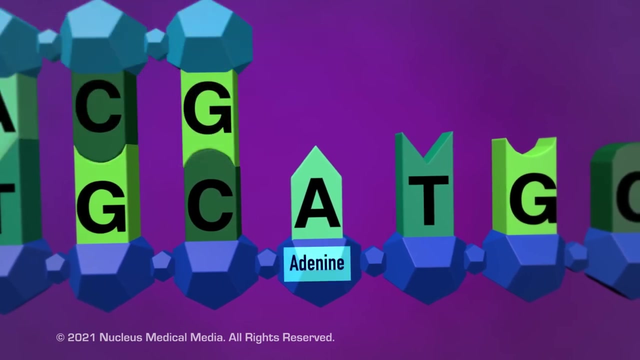 on the template strand, then binds it to a free nucleotide strand containing adenine. This process continues with cytosine binding to guanine and guanine binding with cytosine. Remember, though, RNA will never contain thymine, So whenever RNA polymerase sees adenine, 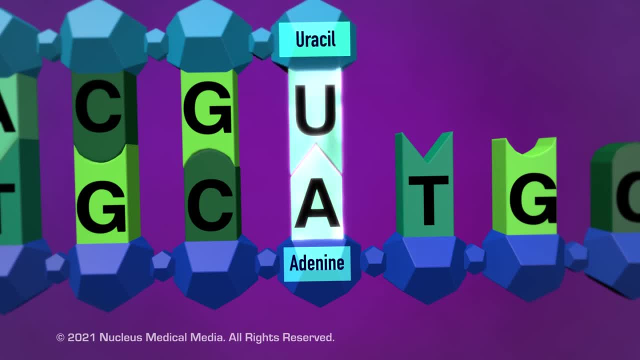 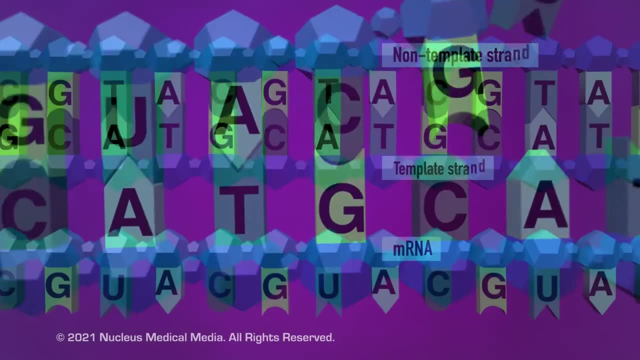 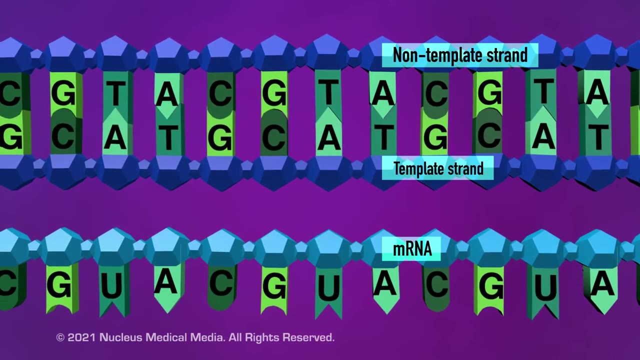 on the DNA template strand. it pairs adenine with uracil By using the template strand of DNA as a guide. the genetic code from the non-template strand of DNA has actually been transcribed into messenger RNA. When transcription is complete, the messenger RNA. 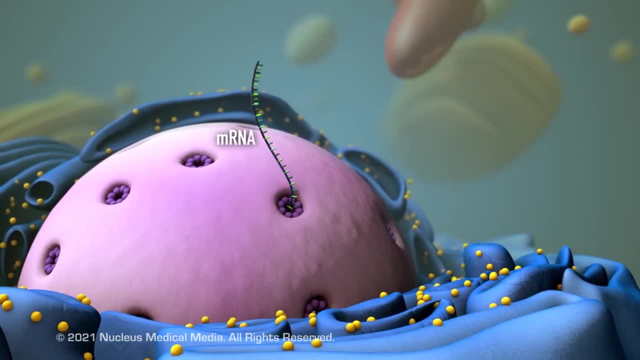 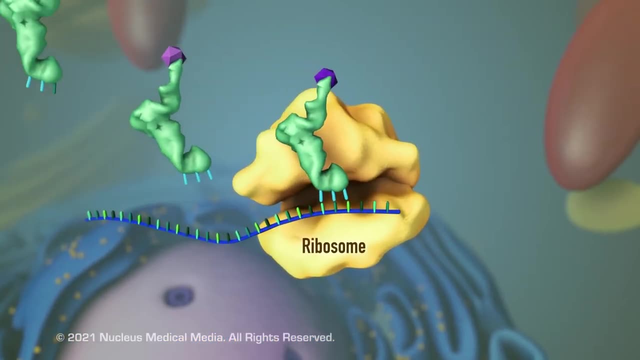 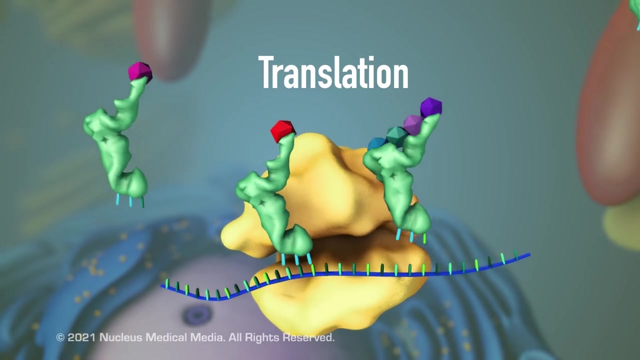 which is small enough to fit through a nuclear pore, takes the genetic code out of the nucleus to the ribosome, the site of protein synthesis. The process of actually building the protein at the ribosome is called translation, which we'll cover in a separate video.